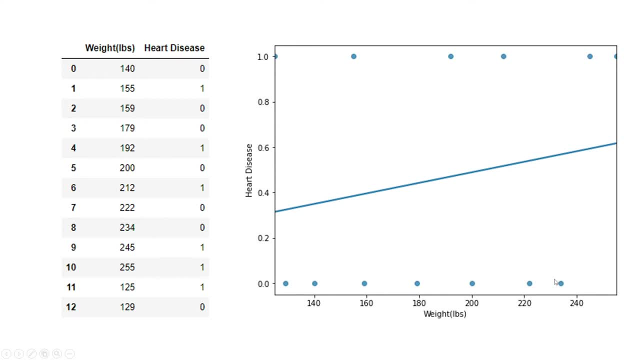 y direction. What happens? all the zero values are here on the zero line and all the 1 values are here on this line, zero or one if we fit a straight line. it actually does not represent these values, these heart disease values, right? so how can we predict this heart disease value, given the weight? 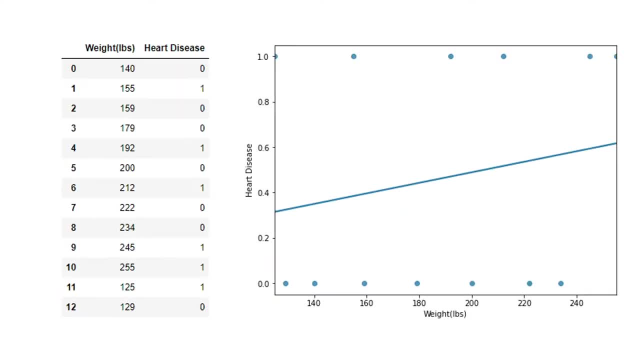 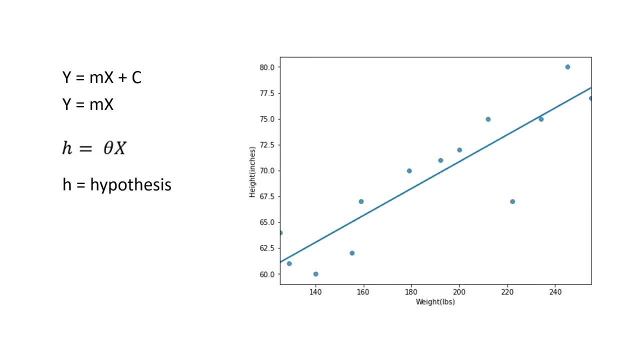 information. this linear regression style is not going to work, so we have to have something different. so, as i mentioned already, this logistic regression also built on linear regression. so we will start from linear regression formula. look: y equals to mx plus c, where m is the slope and c is 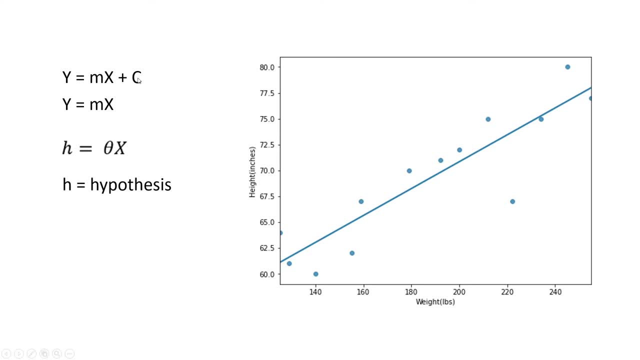 the intercept right now. if we don't use this c or y intercept, we will have y equals to mx. actually, you don't have to ignore c. you can use c as one, but for now we are just going to ignore. in machine learning language we do not call it slope, we actually call it the coefficient of x. 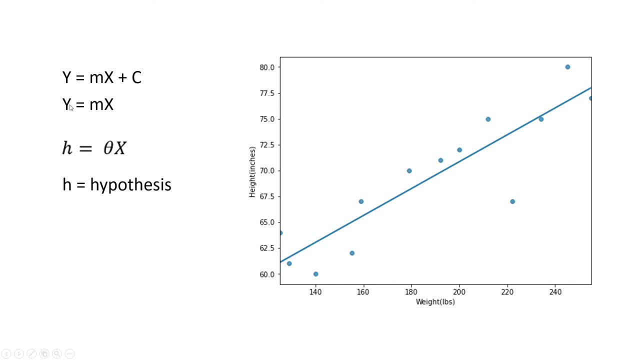 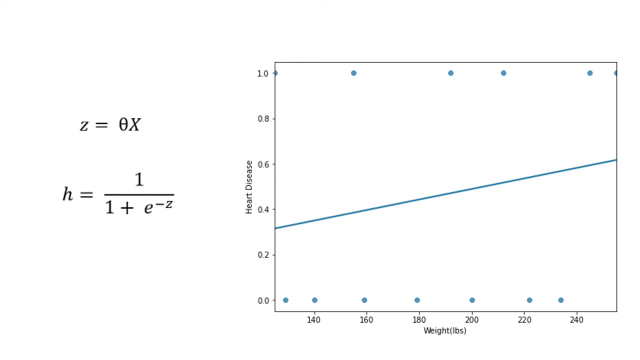 so i am changing m to theta and instead of y I'm using h, because actually we call it hypothesis. So for linear regression the hypothesis is simply the straight line formula. Okay, now what happens when we have logistic regression? In logistic regression the hypothesis formula is different. It's 1 over 1 plus e to the power negative z. 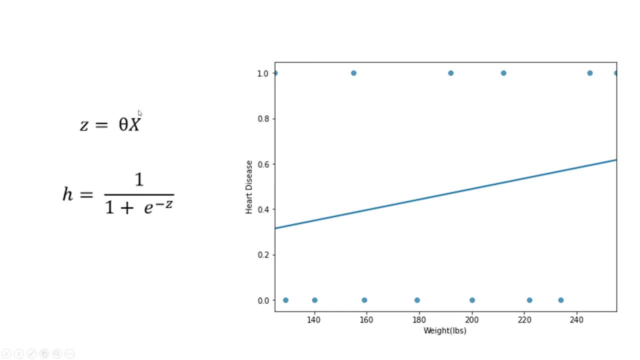 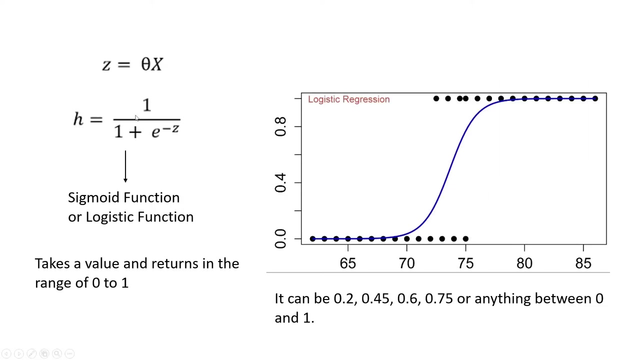 and this z is actually this linear regression formula, theta x. So in logistic regression the hypothesis uses linear regression, but use this function, called as logistic function or sigmoid function, to bring non-linearity, because the straight line is actually not the solution to the logistic regression problem. I already mentioned this function is called sigmoid. 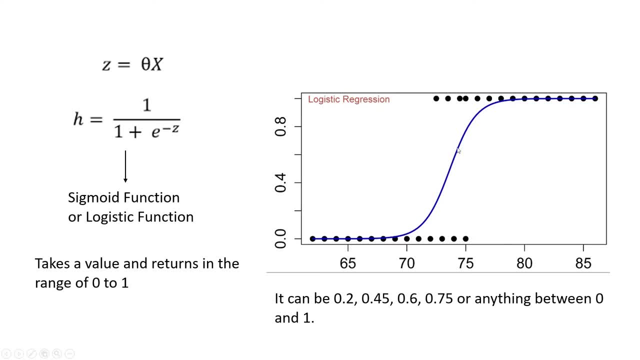 function or logistic function, and the shape of this function is actually like this. this s shape and this function takes a value and returns in the range of 0 to 1.. The value can be 0.2,, 0.45,, 0.65,, 0.8, or anything that is between 0 and 1.. 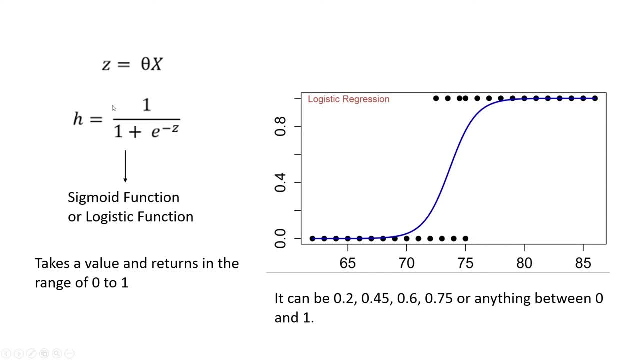 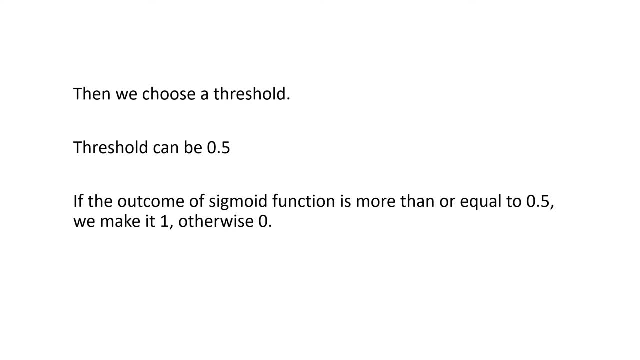 Now, if we have these float values from this hypothesis or from the SIGMET function, how we get 0 and 1 from it? Simply, we choose a threshold. The threshold can be 0.5, or it can be different as well. 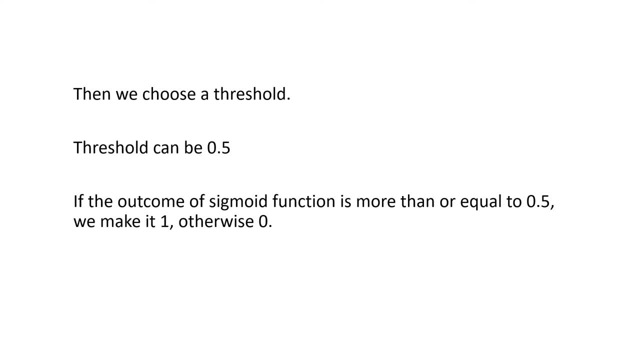 but for now just assume the threshold is 0.5.. If the outcome of SIGMET function is more than or equal to 0.5, we make it 1,, otherwise we make it 0. That's how we get the 0 and 1.. 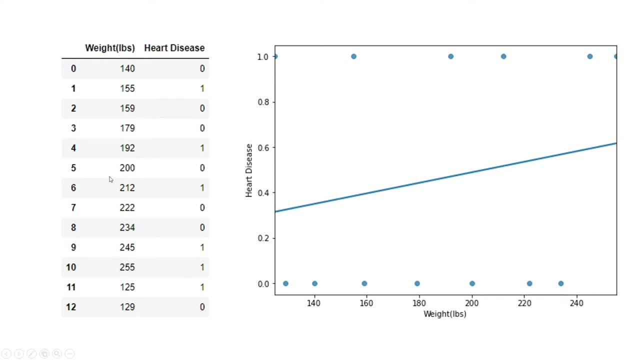 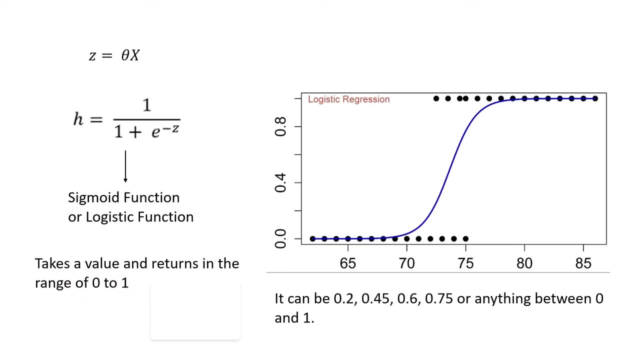 And we use here only weight, one continuous variable. We do not have to have only one variable. Let's go back to this logistic regression formula again. When we had only one variable, the z was theta x. But if we have multiple variables, the z becomes theta 1, x1 plus theta 2, x2. 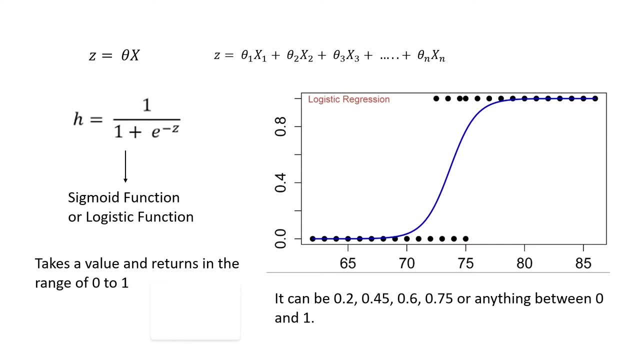 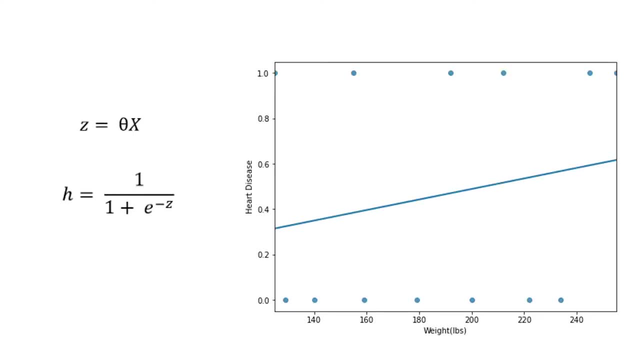 plus theta 3, x3, all the way up to theta n, xn. And as usual the z is used in the SIGMET function: 1 over 1 plus e to the power negative c. That's a very basic and high-level idea of logistic regression. 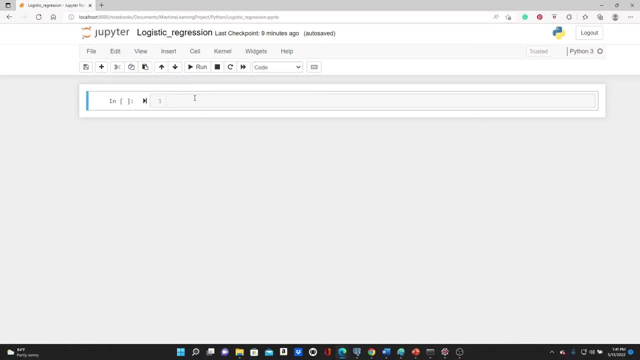 Now let's work on a problem. This is a Jupyter notebook environment. Let's start with importing pandas. pandas is pd, Now the data pdreadcsv. I'm going to use a CSV file, heartcsv. So this data set is from Kaggle and I have the link in the description box below. 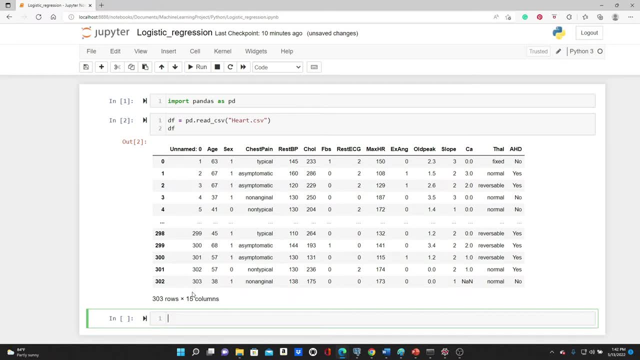 Please feel free to download the data set and follow along. As you can see, we have all this other information: age, sex, chest pain, breast pp and all the other stuff- And at the end I have a hd. This is called heart disease. 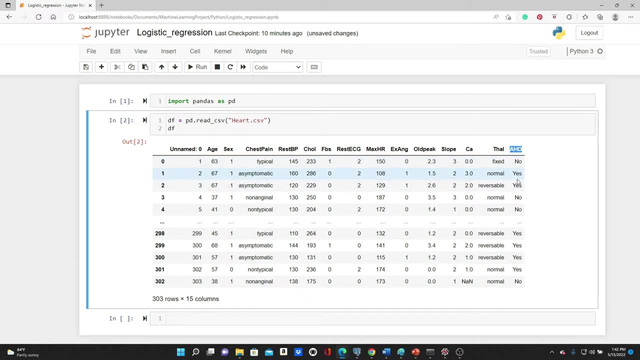 So we have no or yes value. No means there is no heart disease And yes means this person has heart disease. So the task will be to use all these other variables and predict if the person has the heart disease or not having heart disease. 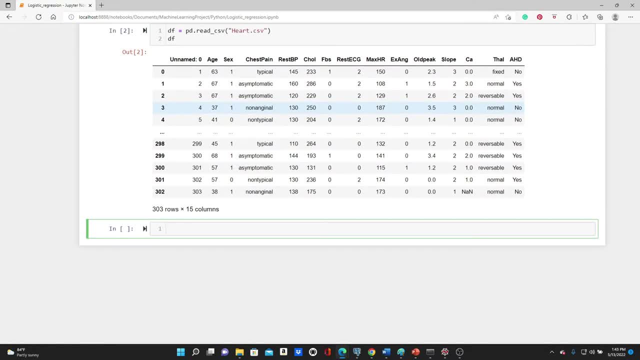 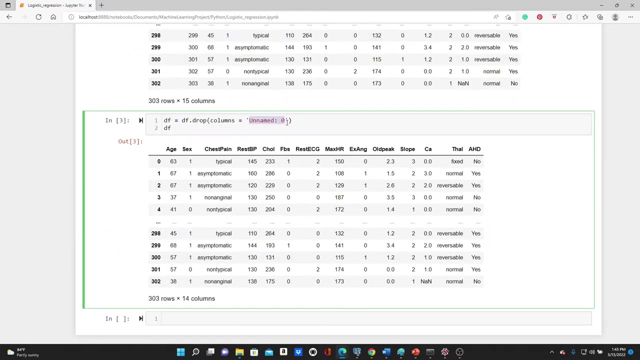 So we need to do some data preparation first. Here we have this column. that's very unnecessary. I'm going to drop it first. dfdrop columns. Now I'm just going to copy and paste this in: This unnamed column is gone. 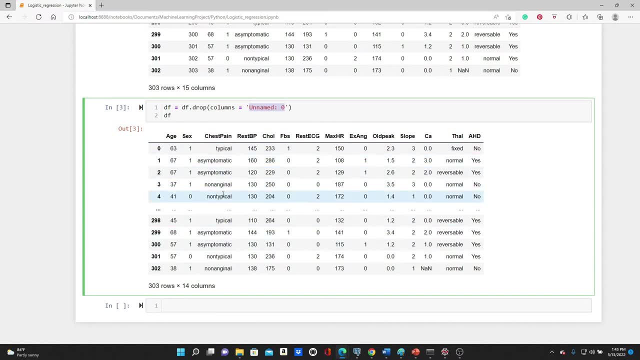 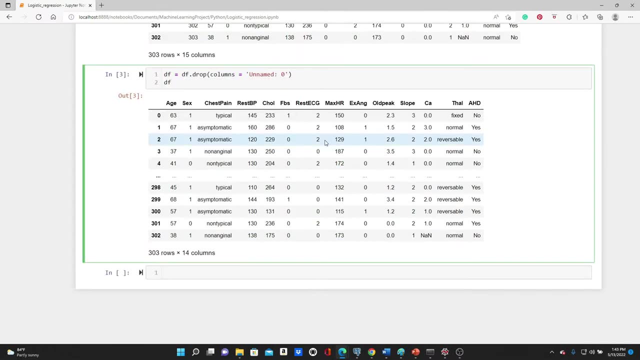 The next is: look, we have this string values: chest pain, thal and ahd. We need to convert them to numeric values because machine learning algorithms do not understand strings, They only want numeric values. Okay, dfdrop, chest pain needs to be in string format. 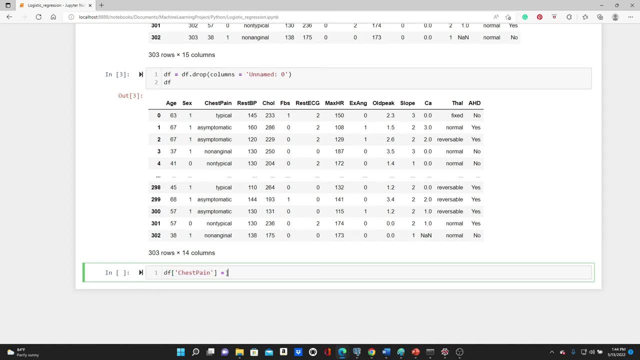 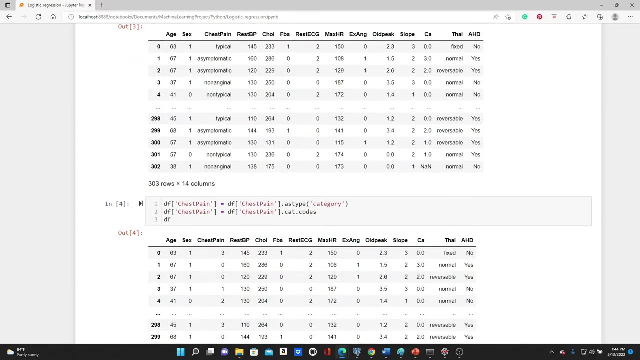 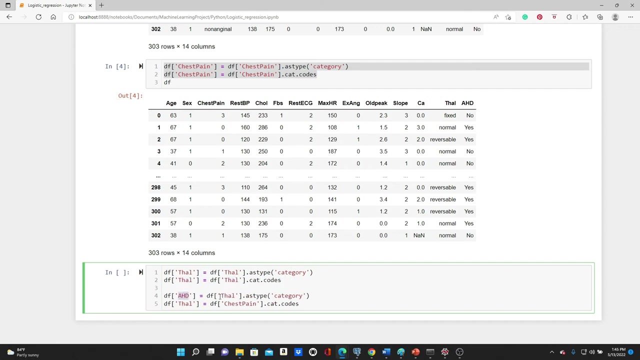 Let's just copy And paste it. Control C, Dot as type category, Then dot cat codes. Let's see df. So the chest pain here, the chest pain string, the chest pain converted into, We have all numeric values right now. 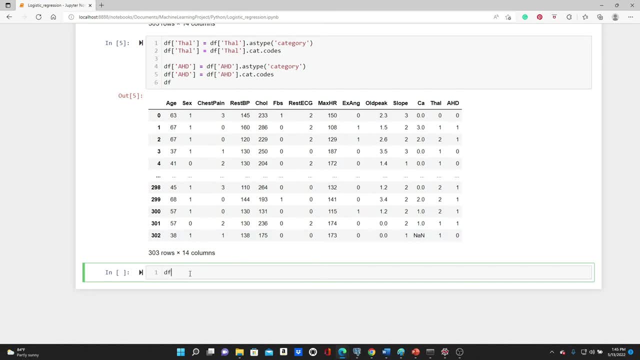 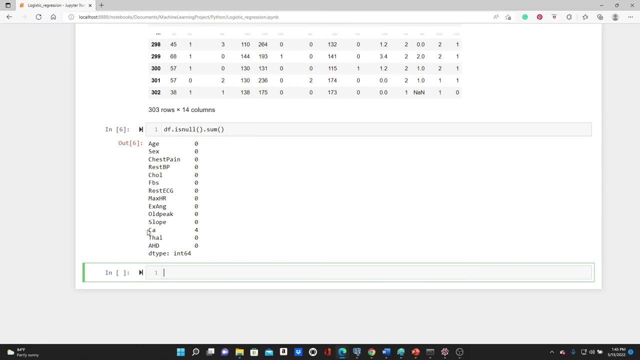 Look, we have one null value here. Let's check how much null value we have. Dot sum, We have only four null values in this C column. Right, We have 303 rows and we have only four rows containing some null values. 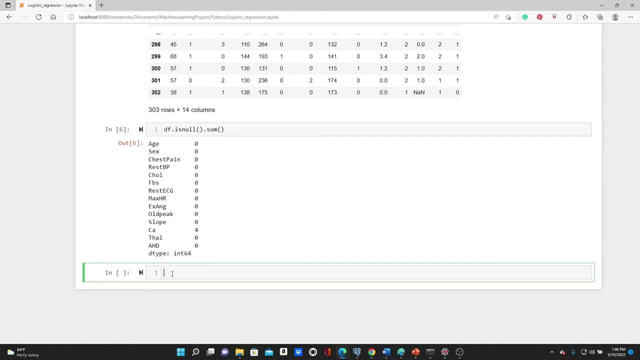 I'm just going to drop them. There are lots of different methods of dealing with null values, but that will be a totally different video. In this video, we are just going to exclude the null values and we only have four rows of null values. 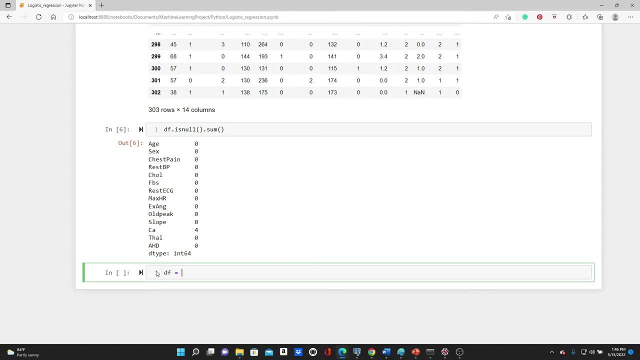 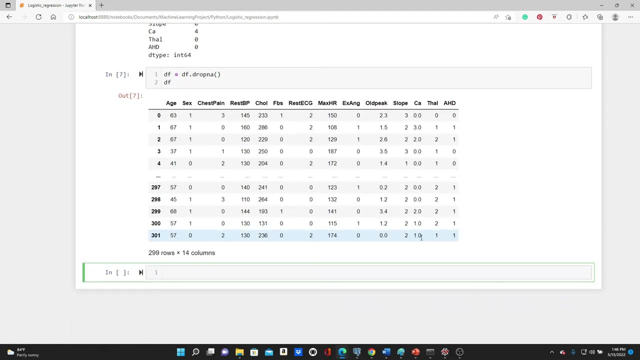 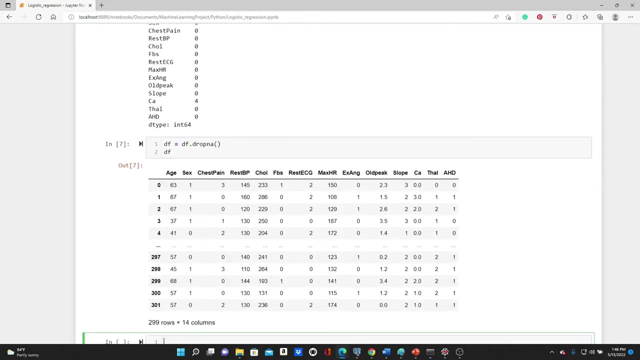 It's going to be easy for us to just avoid them. dfdrop and a. So look we just. we do not have any null values. We have 299 rows before, we have 303 rows, So null values are gone. Data is ready. 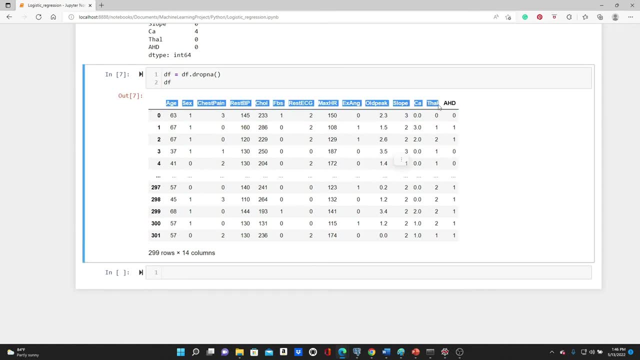 Now look, these are all the variables that are going to be our independent variable, or X input variable, And this is what we are going to predict AHD. So this is going to be our Y. So we're just going to separate X and Y. 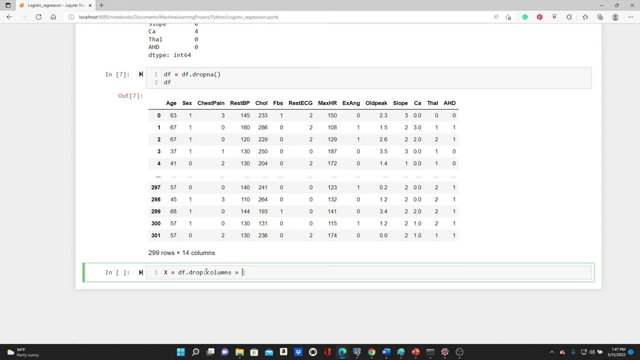 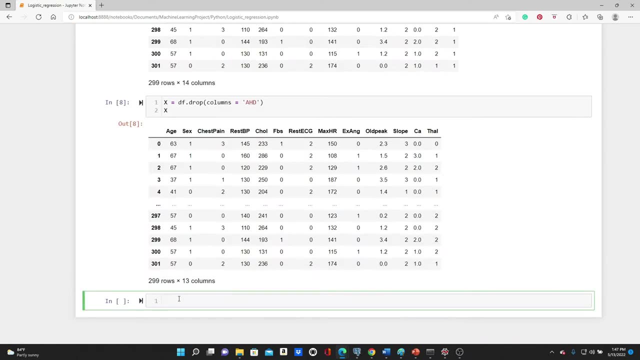 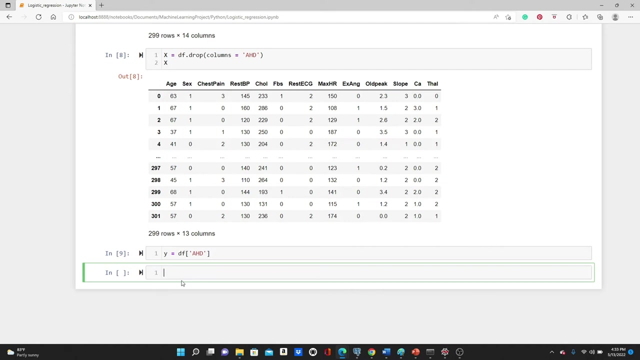 dfdrop columns: AHD. That's going to be our X. We have X, all the values except the AHD, And for Y we have df AHD. Now we will split the data set. We will keep portion of the data set to train the model and portion of the data. 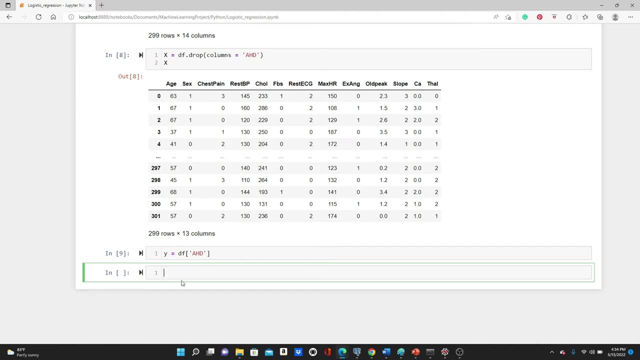 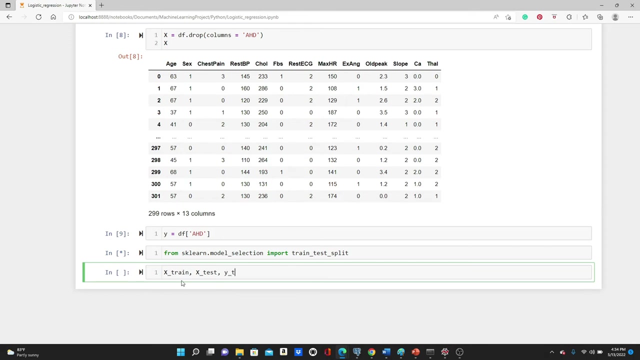 set to test or evaluate the model. We can use train test split method from scikit-learn library, from that From scikit-learnmodel selection Import train test split X train X test Y train. Y test X train. 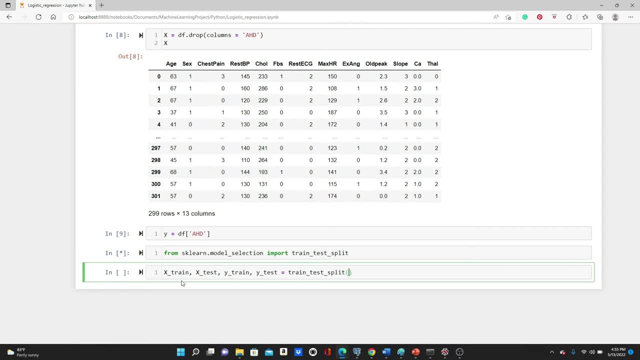 X train test. Split X- Y, Then test size 0.3.. That means we are keeping 30% of the data for testing and 70% of the data for training, And random state is 221.. Random state can be any integer. 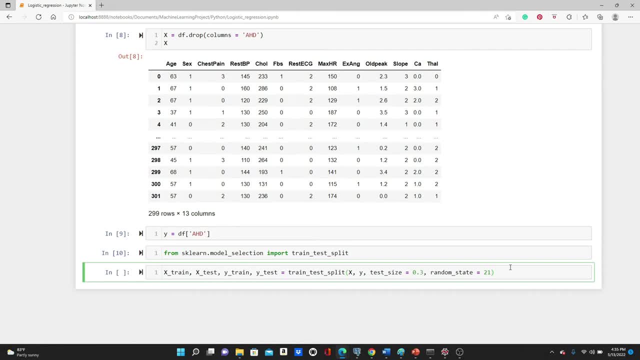 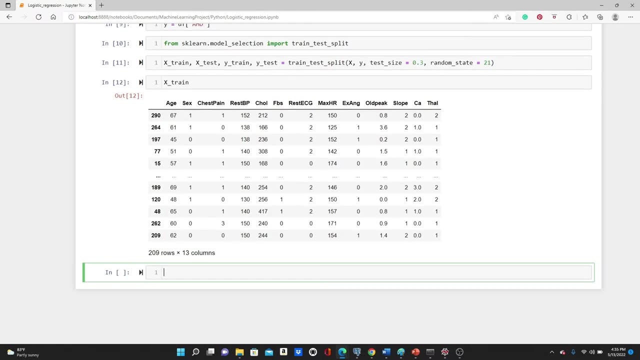 We use random states so that we can regenerate the same train test split if necessary. Let's see the X train now. This is X train. You can see we have 209 rows of data for training and X test. We have 90 rows for testing. 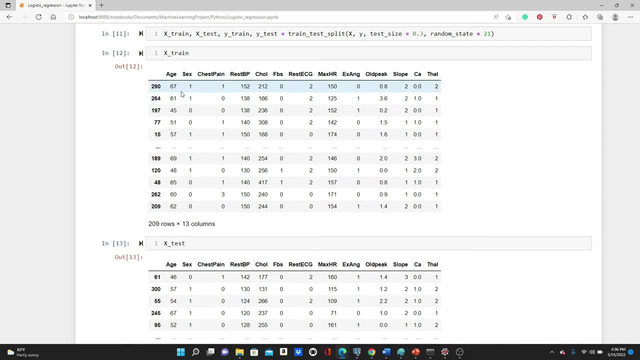 Now look. Look at our training features. Some of the data are 50,, 60,, 30,, 40,, 50, right, And some of the data are 1,, 2, 3 or 0, 1.. 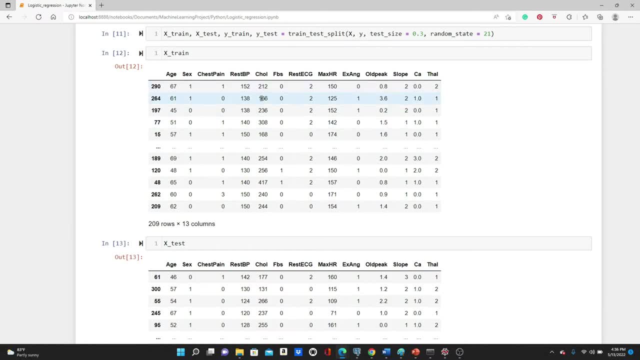 Some of the data are 308,, 200,, 12, 166.. So some data are really big and some data are really small, like 01.. So in this case this bigger data can be a little overpowering If all the data in all the training features are going to be in the same range. 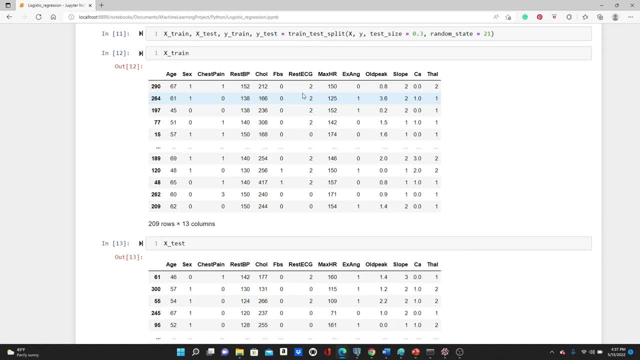 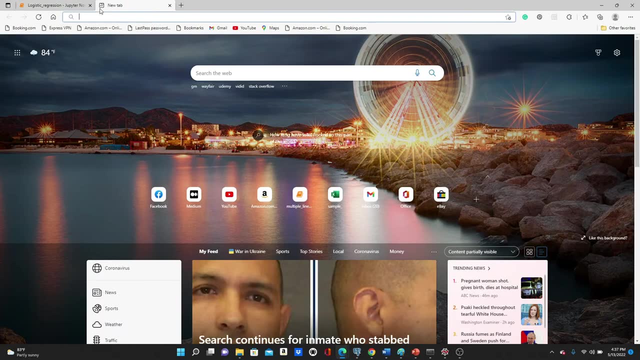 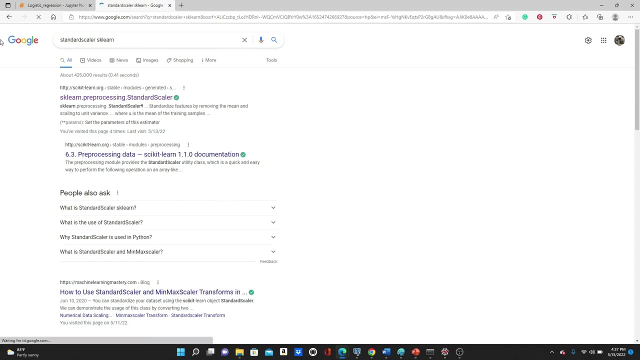 that's going to be good for the training, right? Because no feature is going to be overpowering. So we are going to use a scalar. We will use a standard scalar. I will go and see the Google Standard scalar scikit-learn. 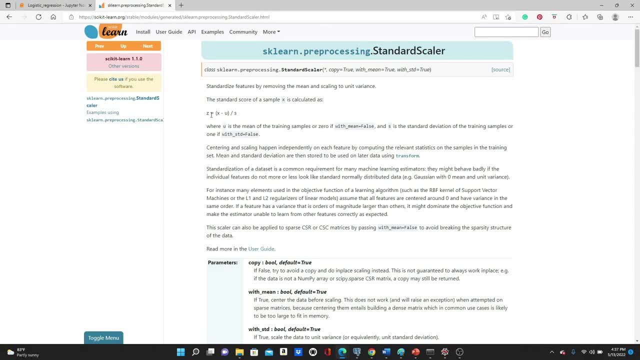 OK, this is standard scalar. You see, it uses this formula, this standardized formula, to scale the data that uses mean and standard deviation. So each and every data uses, like that, data minus mean divided by standard deviation, And that's how it scales the data. 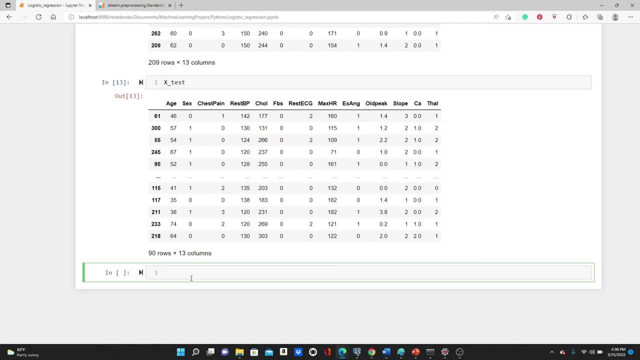 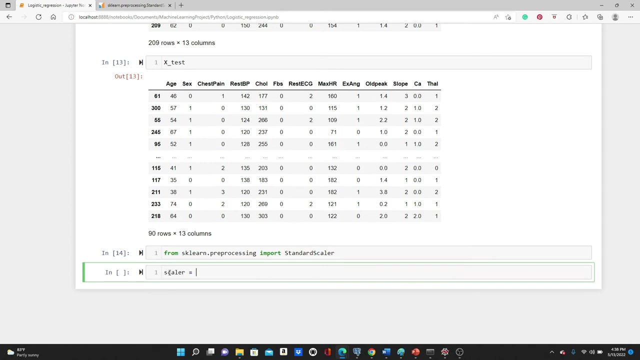 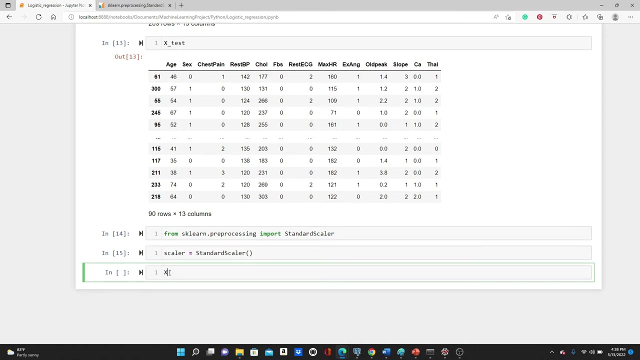 So let's import standard scalar From scikit-learnpreprocessing: import standard scalar, Now scalar, standard scalar, right First with X train, X train scaled, X train scaled. we are going to do scalarfit, transform, OK, fixed, transform X train. 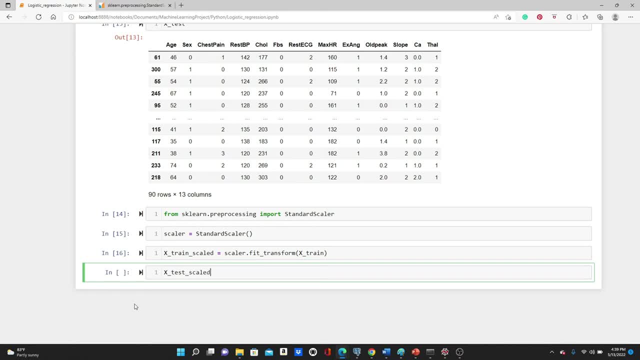 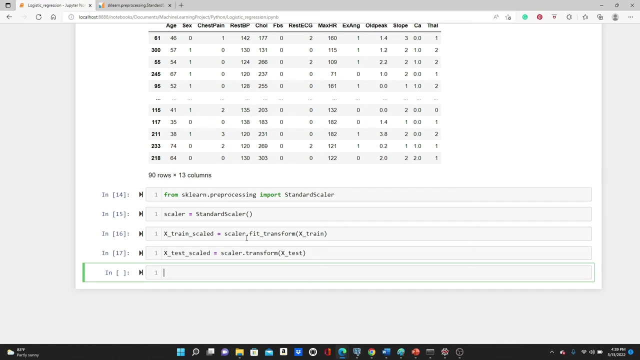 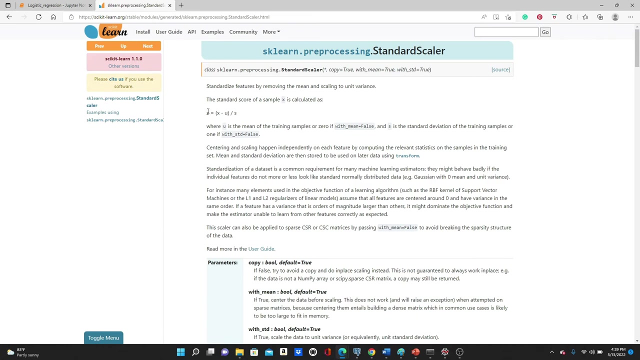 Now X test, scaled Scalartransform only. We're not going to do any fit for X test. It's going to be only transform. Why is that? When we feed the data to the scalar, it calculates the mean and standard deviation of the data. to be able to calculate this Z. 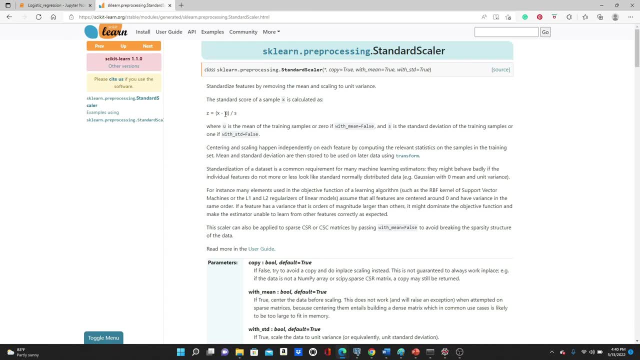 Right, When we feed the data, it calculates the mean and standard deviation, And when we do the transform, it uses this mean and standard deviation and calculates this. Z. We feed the training data so it can use the training data to calculate these parameters- the standard deviation and mean- and then it can use it to transform the data. 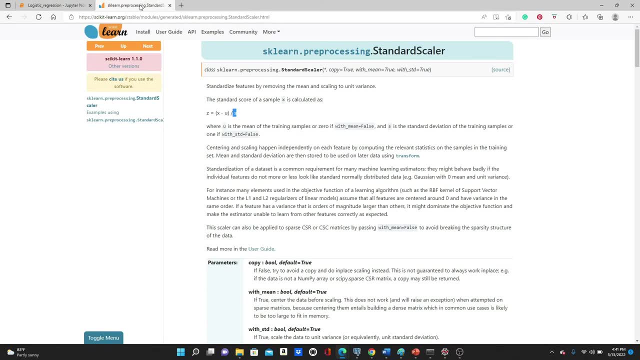 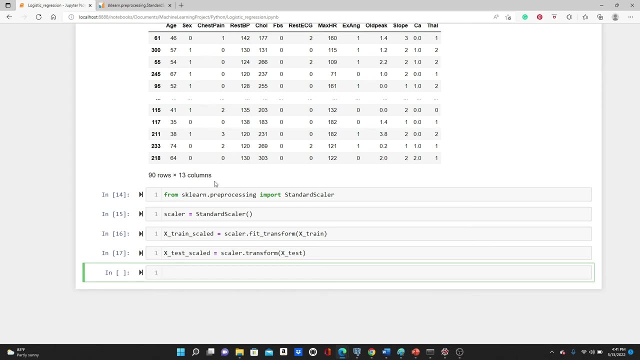 But we don't want to feed the test data to the scalar because we don't want our model to know the mean and standard division of test data. We will keep strictly the test data for evaluation purpose. We don't want our model to know any information about the test data. Okay, we'll simply transform it using this feed data. 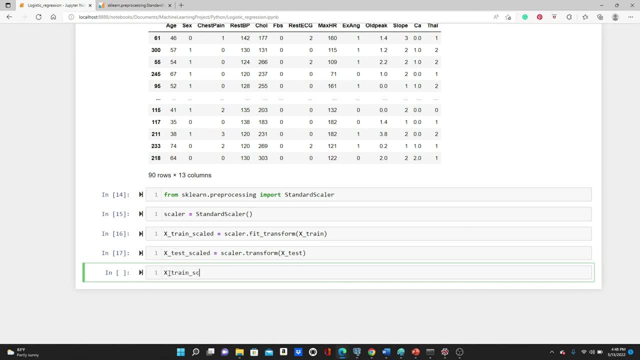 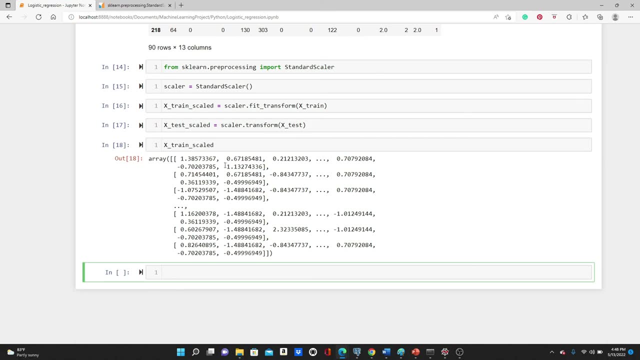 from the training data. Let's check how our scale data set or scale features look. Look, this is how our scale features look. Look, all of them are pretty much similar range. It just transformed into the two-dimensional array instead of data frame format. Our x test scale also. 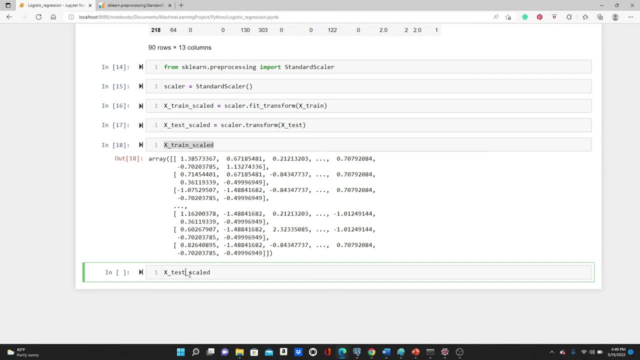 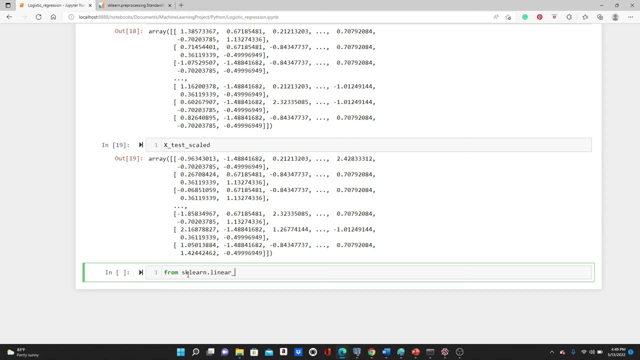 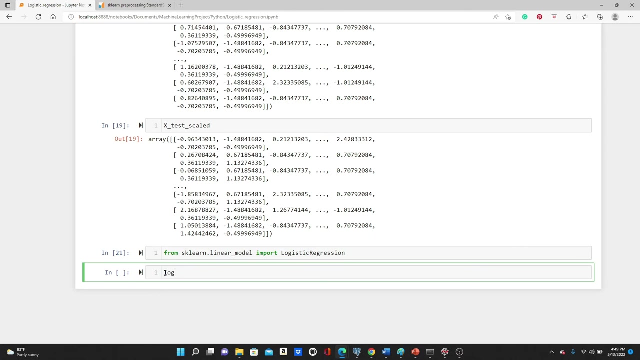 became this same form. Now we will import the logistic regression from sklearnlinear model. Okay, import logistic regression. Oh sorry, regression. So log reg logistic regression. I will use random state zero if we want to recreate this same model. dot feed: We're going to feed our scaled training. 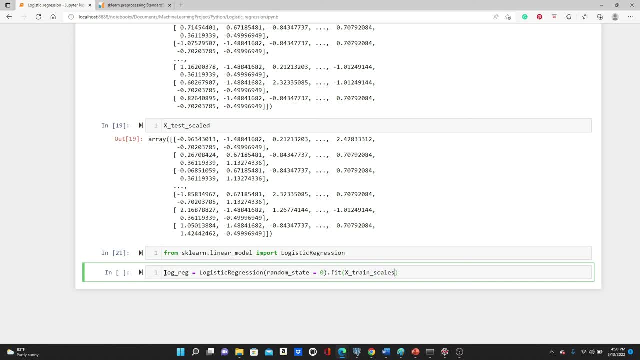 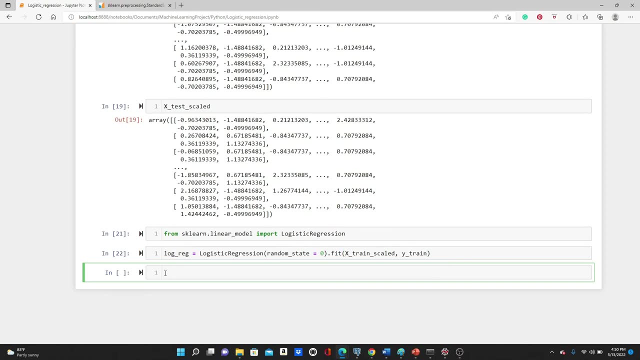 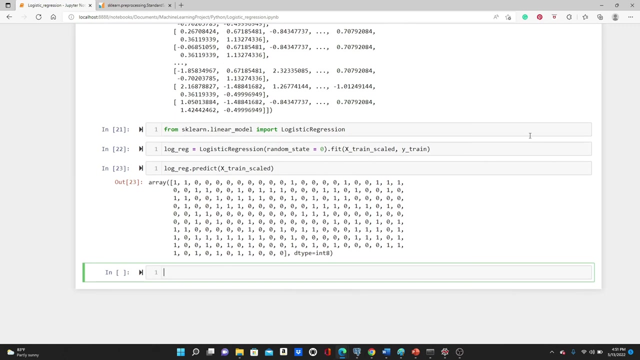 data: X train scaled and the label y train. So the model training is done. Now we should check if it can predict. Log reg dot predict: If I put x train scaled, it should give me y train. Look, it's the y train. zero and one value right. 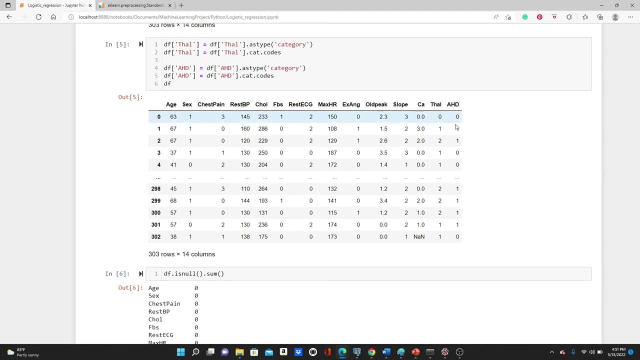 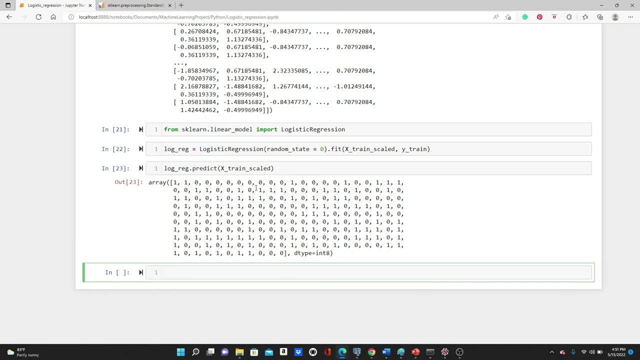 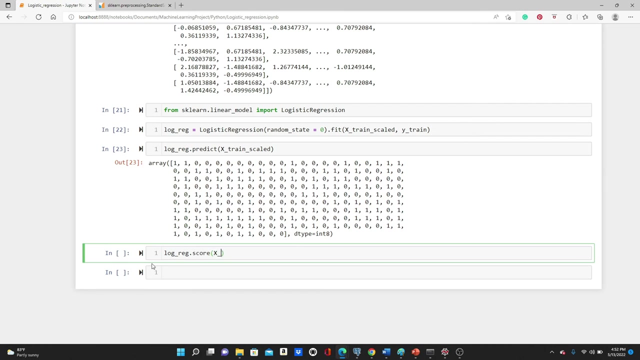 Let's check. Look our y value or this heart disease data. it was zero and one, So these are zero and one value. How accurate these output values are? Log reg dot score x a crane skein y train. So it says 87% correct. That means 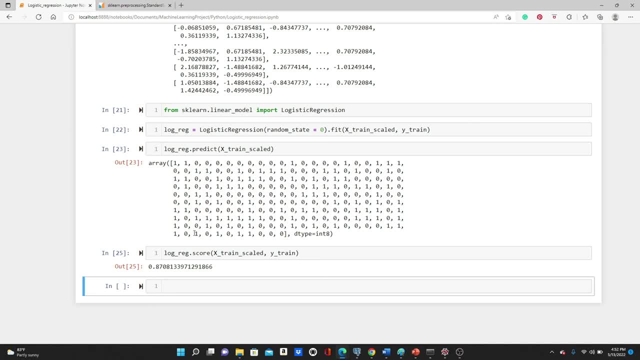 87% of this output values are actually accurate. Okay, this is on the training data, and we already fit the training data to the model, and our model already know the training data. So well, now let's check if it can generalize or it can predict from test data as well. test 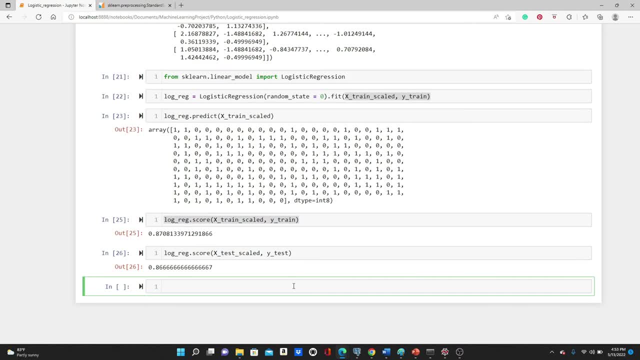 and give y test, it shows that 87- almost 87- percent of the time it can predict the test data as well. so our model is pretty strong. you should always check accuracy for training data and test data, both. if the accuracy for training data and test data is really different, like if it's 87 and it's 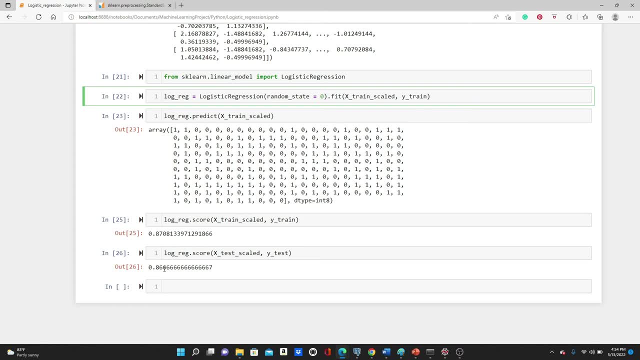 uh, on test data is 67. the model is not good at all. we want it good on both training and testing data. let's check if we can improve this model using some more parameters. so let's take it and make it log red one, and i'm going to use some more parameters here. 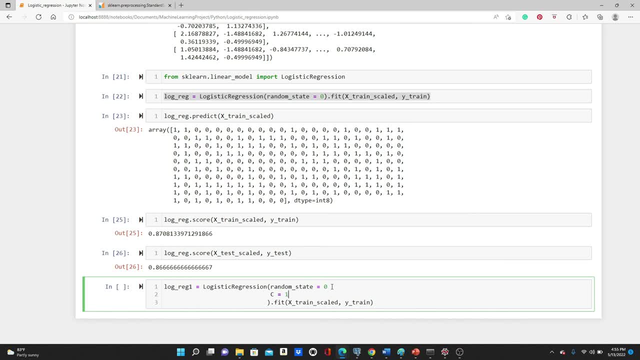 number one parameter is i'm going to use c. c is one. c is a regularization parameter that penalizes the extreme values. that should improve the model. okay, now i will use the fit intercept. true, remember the intercept here. in the beginning, in linear regression, we had mx plus c and 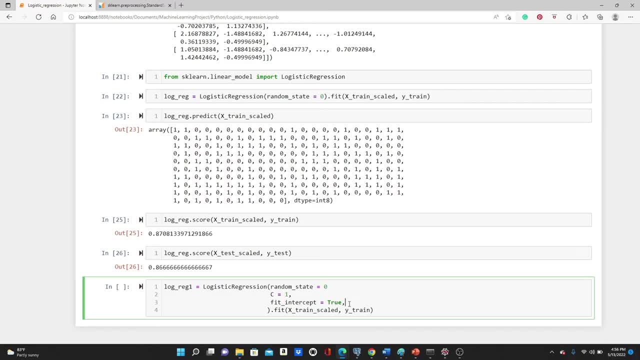 we said we can ignore the intercept, but we can use it. so here is the option where we can enter the intercept and then we can use it in the linear regression. so we can use it in the linear, actually use the intercept. all right, let's check how good it does. oh sorry, i missed a comma here. 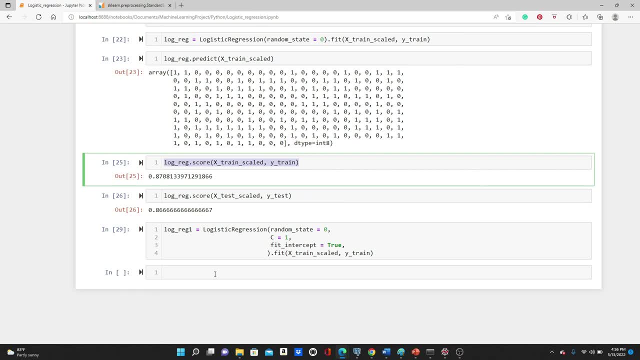 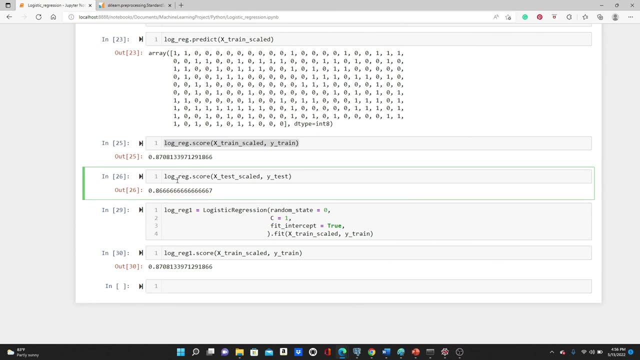 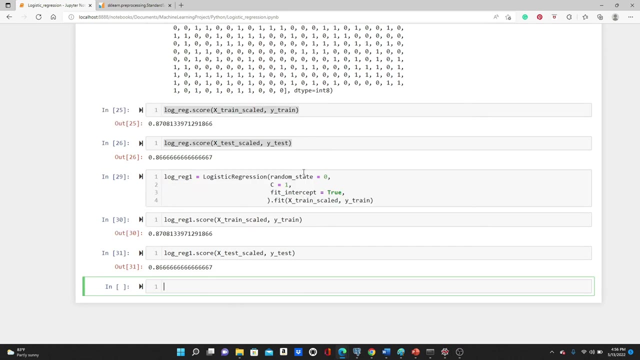 so now grab one. let's check the score. now log red one one. you can see it's still 87. it didn't really improve much. and now grab one. all right, here also it didn't improve much. let's check if we can use a different c, and it can have. 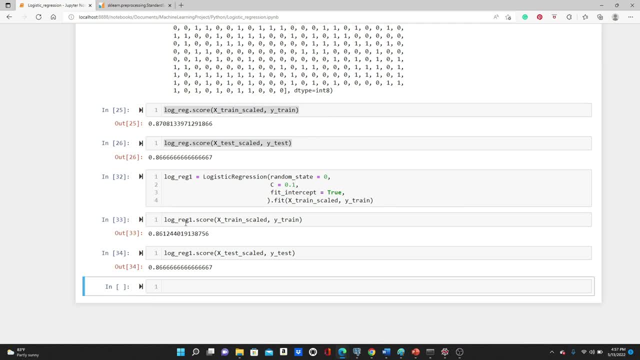 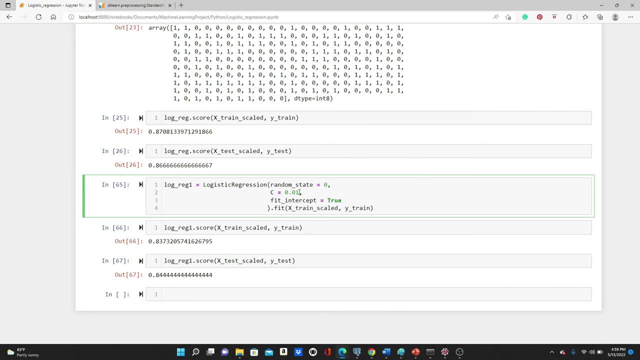 0.1. okay, it didn't improve at all, especially in training set. it kind of lowered the value a little bit, but in testing data it's exactly the same as before. now let's do 0.01. so changing the c and feed intercept didn't do any good now. 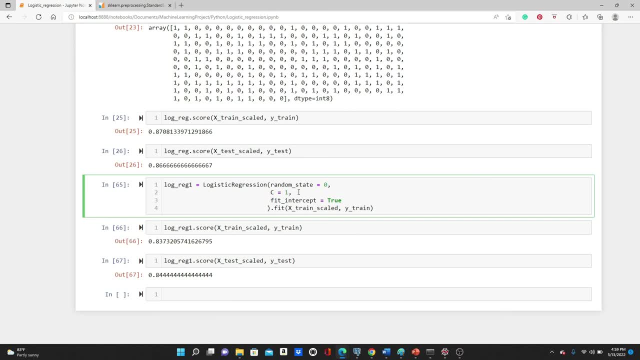 if we go back to our original c1, one is actually the default c, but if you don't give any c value, it uses one automatically. so that's the best. as we checked for this particular data set. changing these parameters didn't do any good, but each data set is different, so the model performs differently. 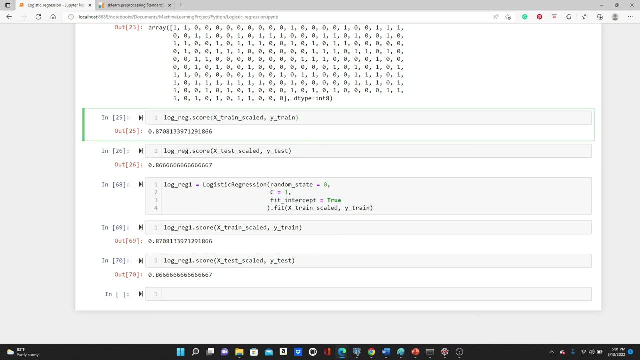 for a different data set in your real life projects. if you do not get good accuracy score like this, like 87 percent or 86 percent, you should try changing the parameters, the c value, feed, intercept, etc. lots of time that improves the model performance significantly. so for this model it didn't change, but i wanted to introduce the.